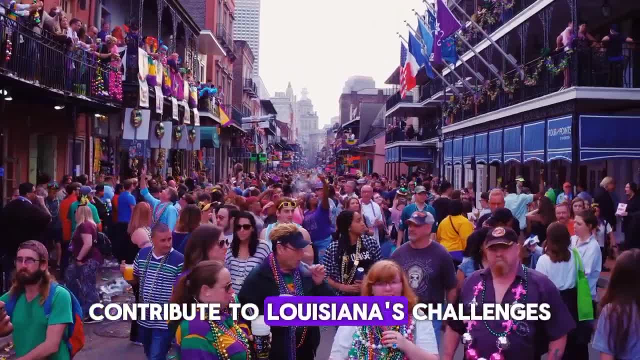 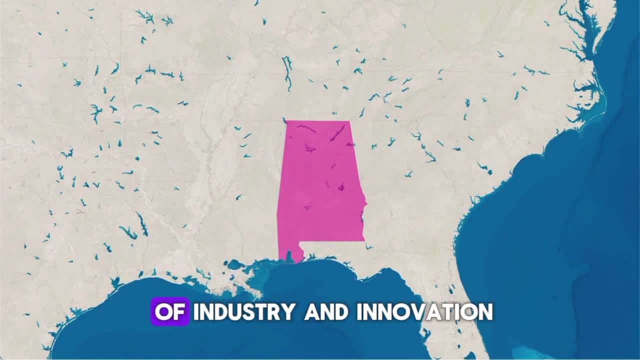 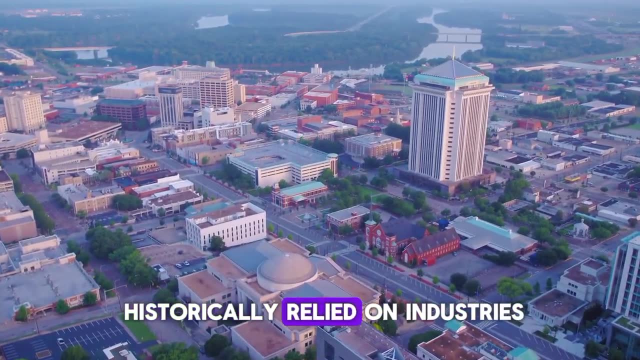 inadequate health care and education systems further contribute to Louisiana's challenges in retaining its population. 4. Alabama, Once a hub of industry and innovation, Alabama has faced population decline in recent years. The state's economy has historically relied on industries like manufacturing agriculture. 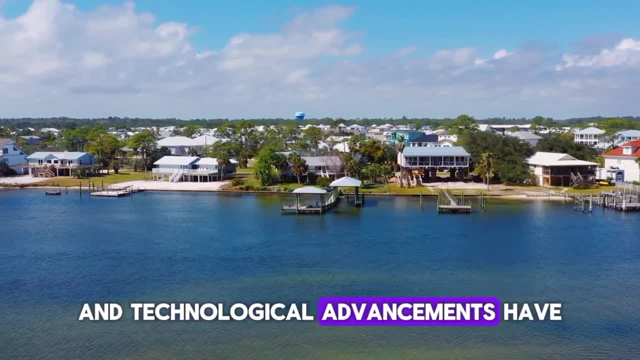 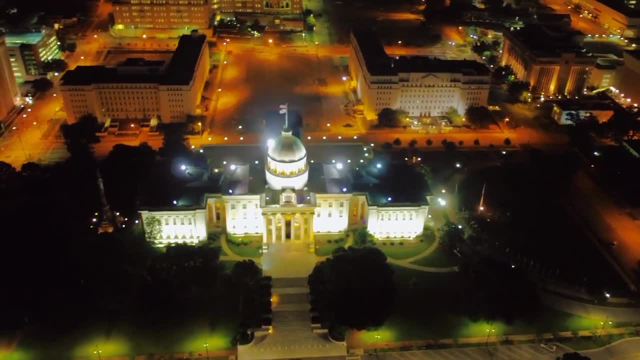 and aerospace, but globalization and technological advancements have led to job losses and economic stagnation. High poverty rates, limited access to health care and education, and concerns about infrastructure and government corruption drive many of Louisiana's population decline. 4. Alabama- Alabama's economy has historically relied on industries like manufacturing, agriculture. 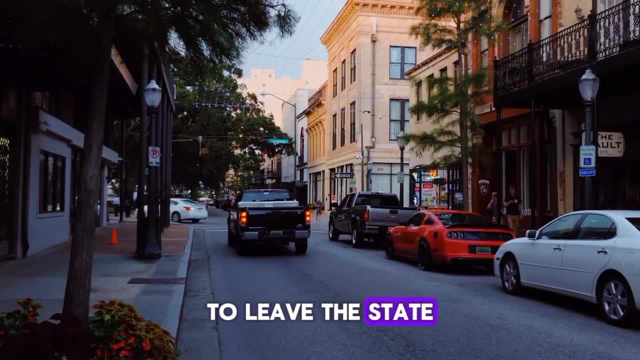 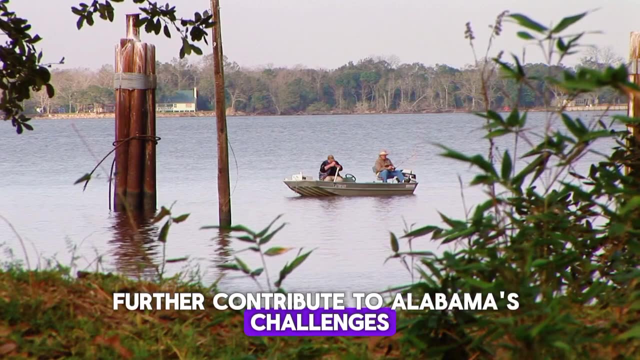 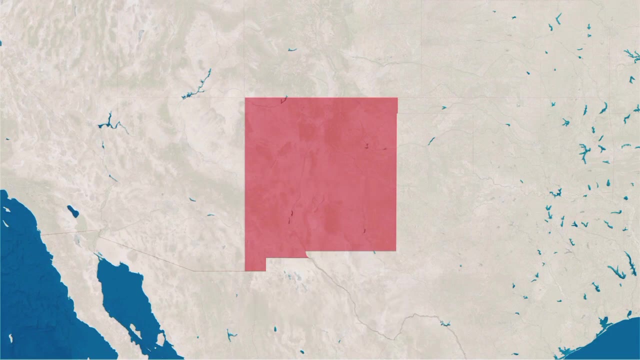 and food. This was not the case for a long time. Alabama is still one of the only states in the United States to have an expense-free economy. Alabama has praying. Alabama's economy is a great example of power, wealth and economic prosperity. Alabama has accomplished its needs. 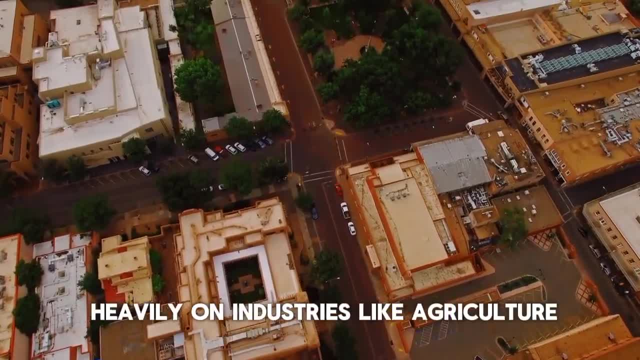 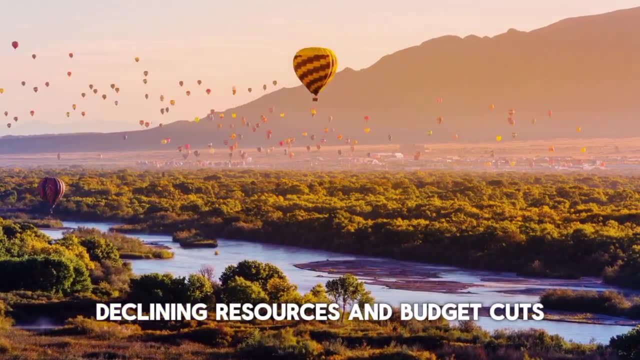 both economically and clinically. The state's economy relies heavily on industries like agriculture, agriculture and food. Alabama is also one of the largestZlaman economy in agriculture, mining and government, which have faced difficulties such as droughts, declining resources and budget cuts, Limited job opportunities, high poverty rates. 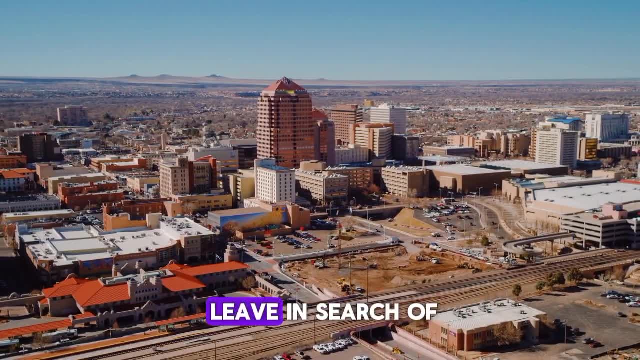 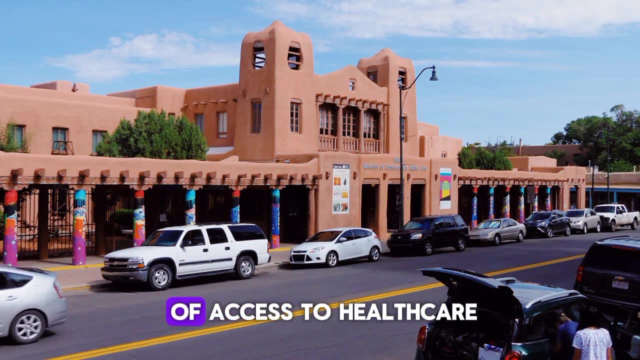 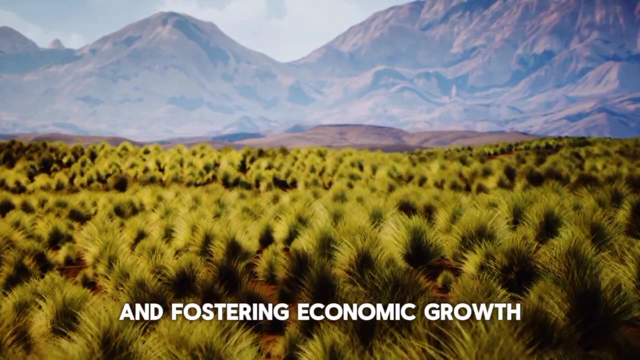 and inadequate infrastructure drive many residents to leave in search of better prospects elsewhere. Additionally, issues such as crime, substance abuse and lack of access to health care further exacerbate New Mexico's challenges in retaining its population and fostering economic growth. 6. Illinois. 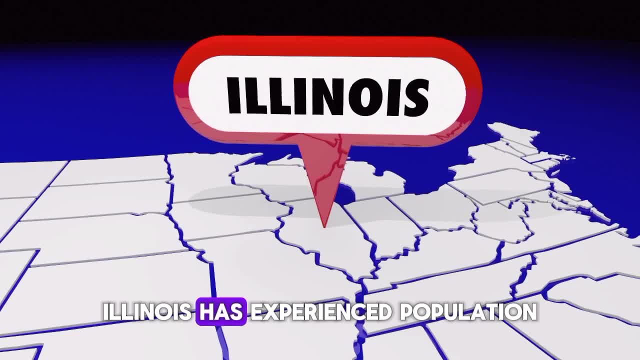 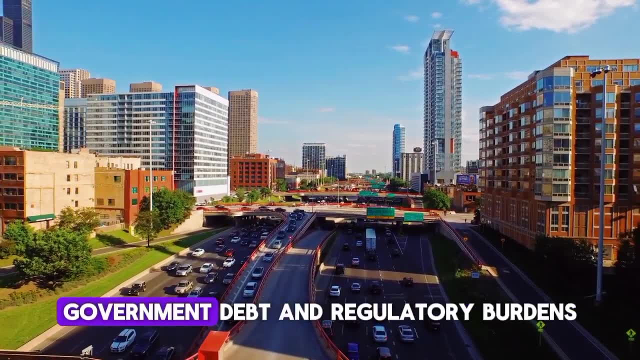 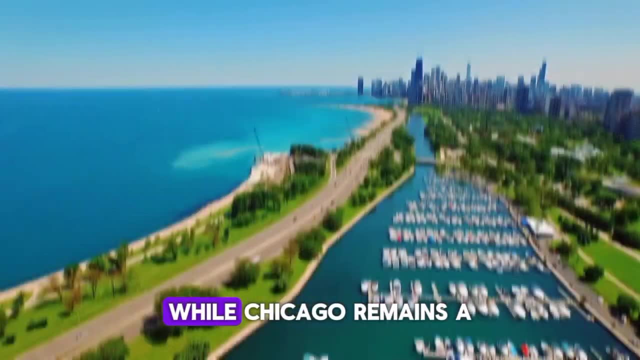 Once a thriving center of commerce and industry, Illinois has experienced population decline in recent years. The state's economy faces challenges such as high taxes, government debt and regulatory burdens which drive businesses and residents to leave for more favorable environments. While Chicago remains a major economic hub, many areas outside of the city struggle with. 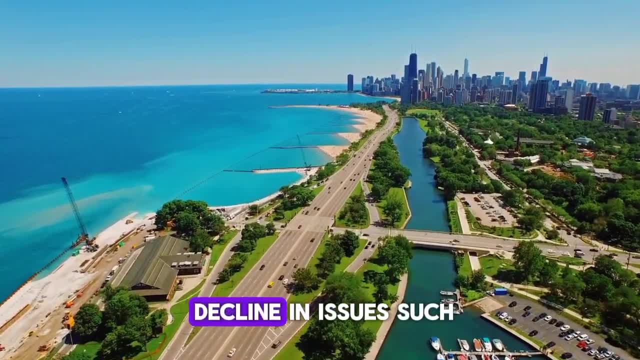 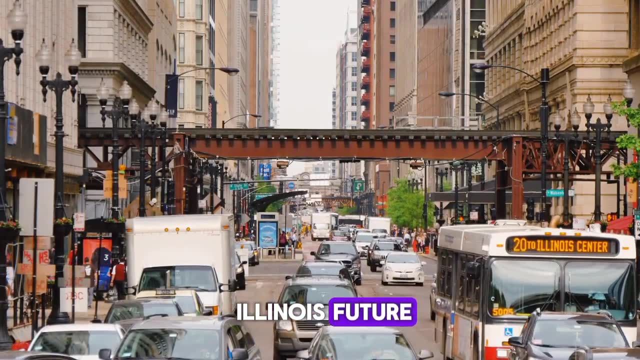 economic stagnation, job losses and population decline. Issues such as crime, substance abuse and lack of access to health care, crime, corruption and political gridlock further undermine confidence in Illinois' future, exacerbating its challenges in retaining its population and stimulating economic growth. 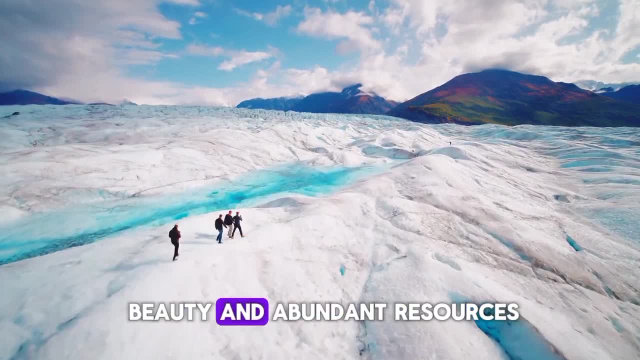 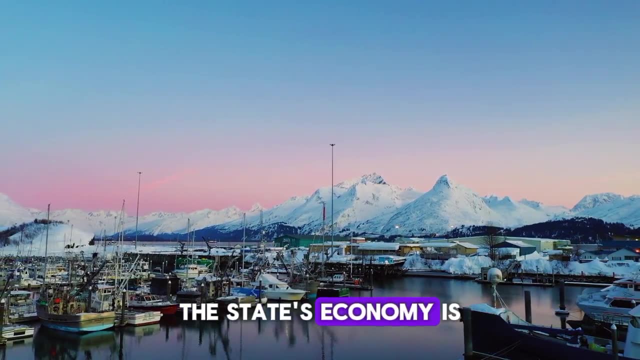 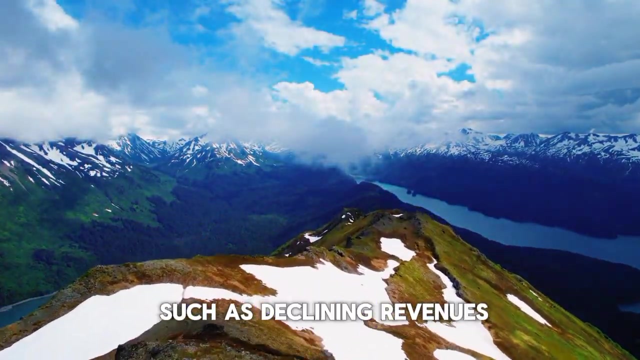 7. Alaska. Known for its natural beauty and abundant resources, Alaska faces population decline due to economic and environmental factors. The state's economy is heavily reliant on industries like oil and gas, fishing and tourism, which have faced challenges such as declining revenues. 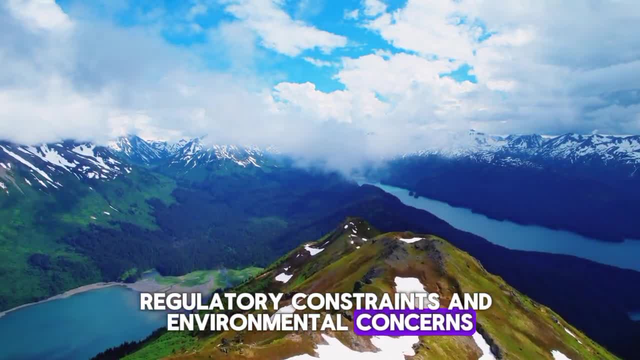 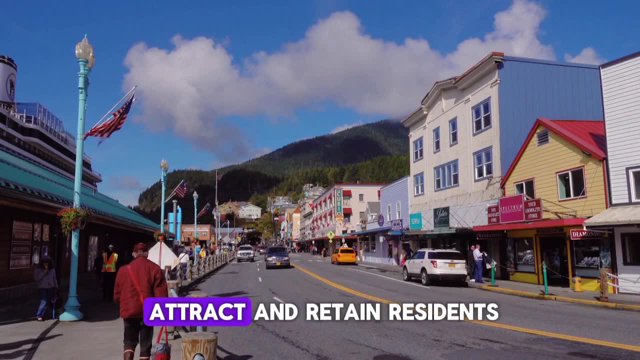 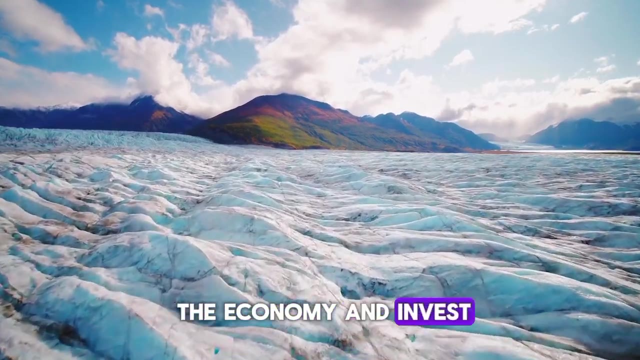 regulatory constraints and environmental concerns. Additionally, Alaska's remote location, harsh climate and limited infrastructure make it difficult to attract and retain residents, particularly young people and families. Despite efforts to diversify the economy and invest in infrastructure, the state continues to face challenges in stimulating population. 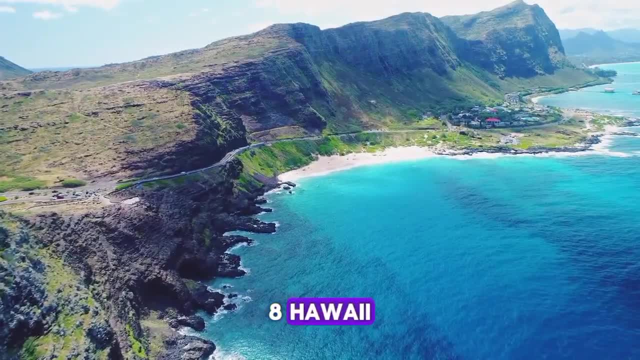 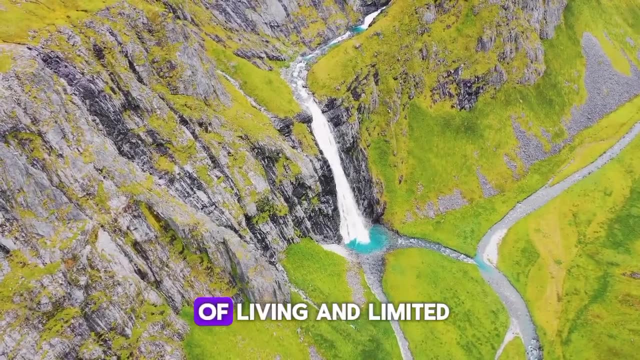 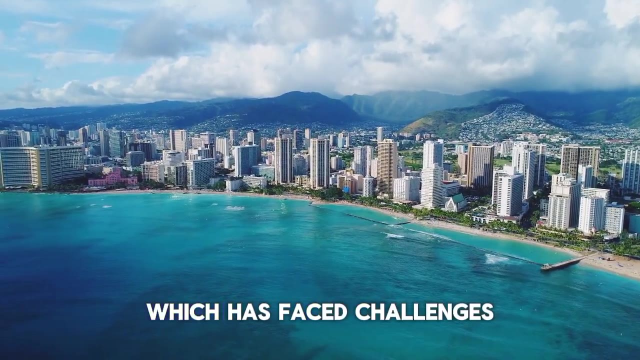 growth and economic development. 8. Hawaii, Despite its setting and strong tourism industry. 5. Hawaii: The state's economic growth and production struggles with population decline due to high costs of living and limited economic opportunities. The state's economy relies heavily on tourism, which has faced challenges such as fluctuating 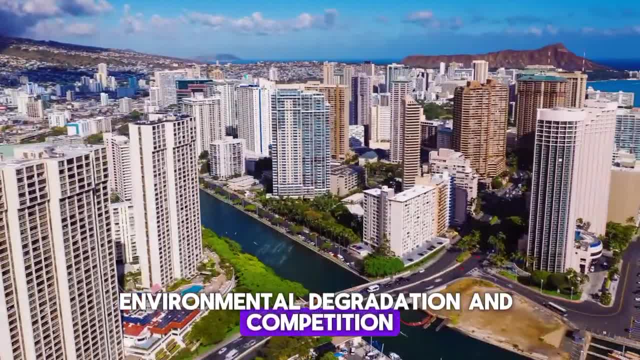 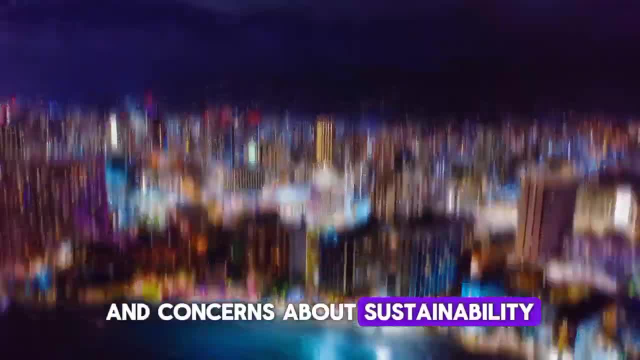 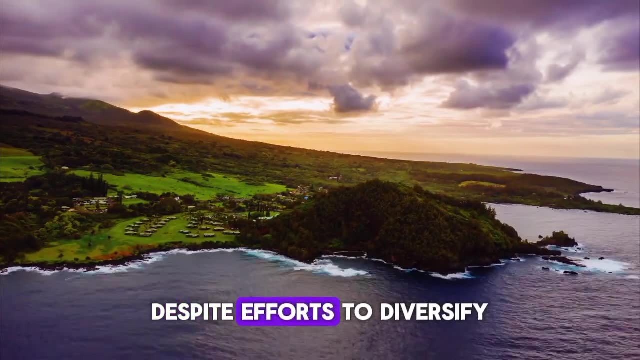 demand, environmental degradation and competition from other destinations. High housing costs, limited job opportunities and concerns about sustainability drive many residents to leave the state in search of more affordable and stable living conditions. Despite efforts to diversify the economy and promote sustainable development, Hawaii continues to face challenges in retaining 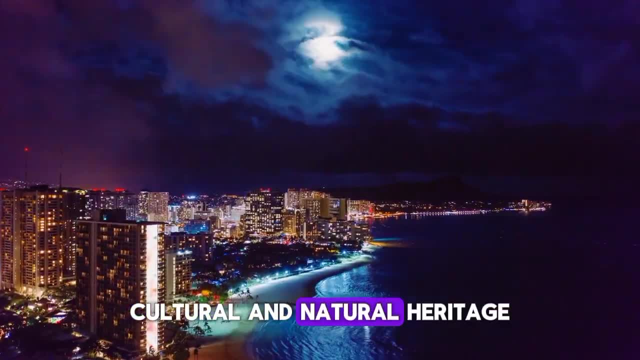 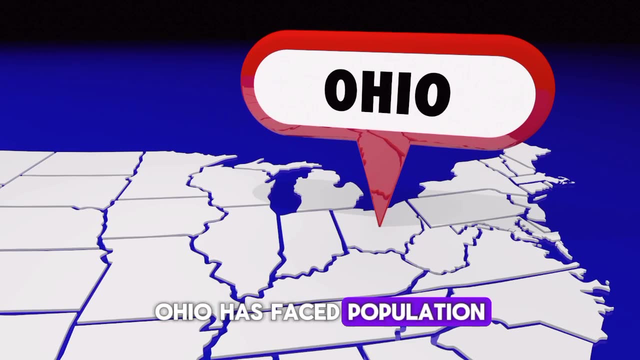 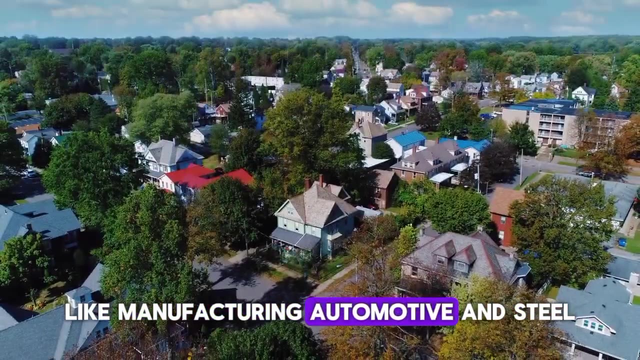 its population and preserving its unique cultural and natural heritage. 9. Ohio: Once a manufacturing powerhouse, Ohio has faced population decline in recent years. The state's economy has historically relied on industries like manufacturing, automotive and steel, which have faced challenges such as globalization, automation and outsourcing. 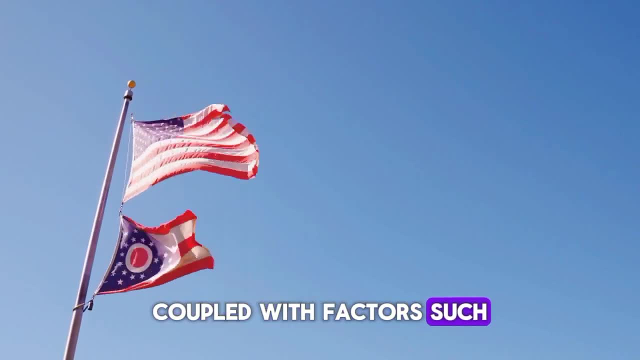 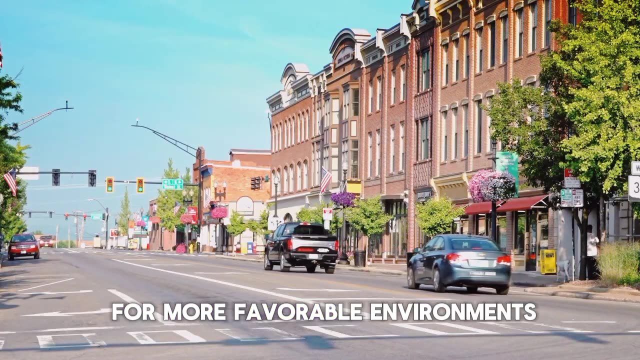 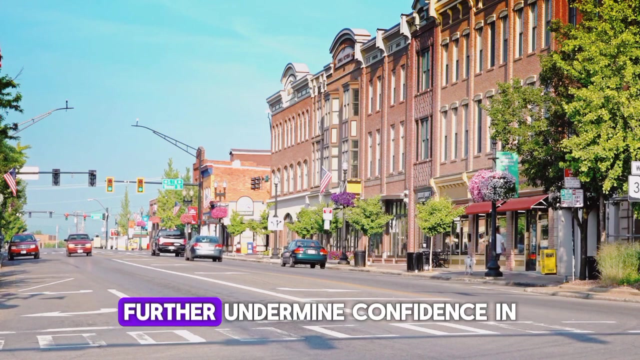 Job line Losses in these sectors, coupled with factors such as high taxes, government debt and regulatory burdens, drive businesses and residents to leave for more favorable environments. Additionally, issues such as opioid addiction, poverty and inadequate infrastructure further undermine confidence in Ohio's future, exacerbating its challenges in retaining its population.